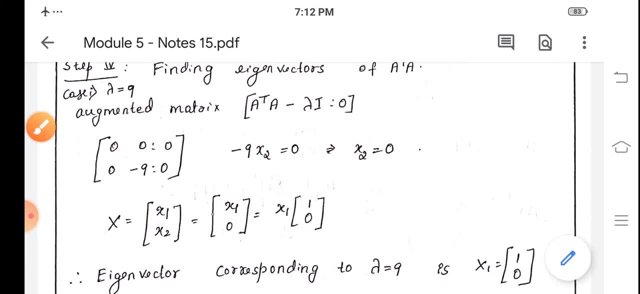 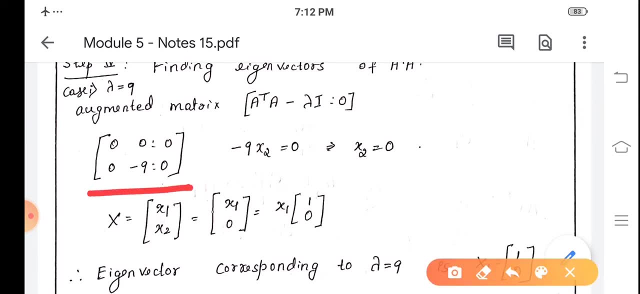 We write the augmented matrix as A transpose: A minus lambda I, 0.. Since lambda equal to 9, augmented matrix is 0: 0, 0, 0 minus 9, 0.. Now we can write the system of equation that is minus 9, x 2 equal to 0, that gives x 2 equal to 0. 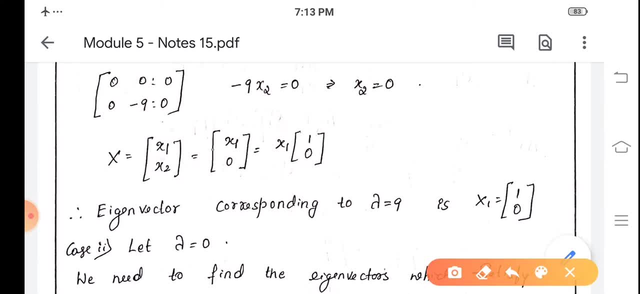 Now we can take column vector x as x 1, x 2, and since x 2 is 0, it is x 1: 0 or x 1 into 1: 0.. Now eigenvector corresponding to lambda equal to 9 is x 1 equal to 1: 0. 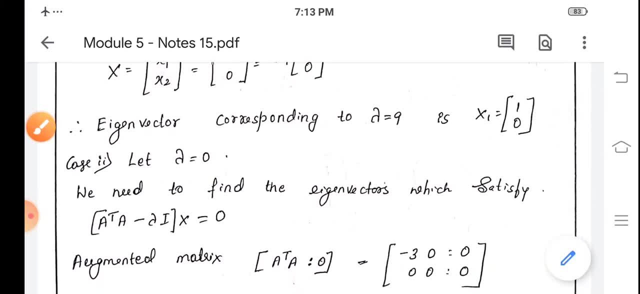 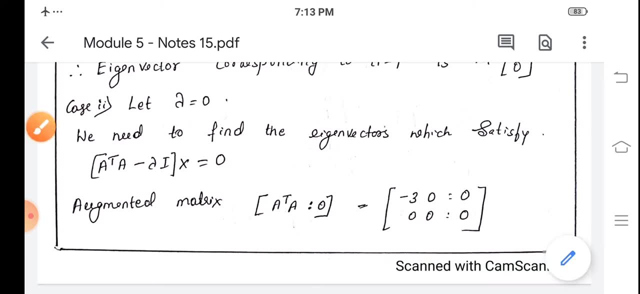 Next we find the eigenvector for lambda equal to 0.. Here we need to find the eigenvector which satisfy A. transpose A minus lambda I into x, 1 x 2.. So we obtain the algorithm which suffices��니다. 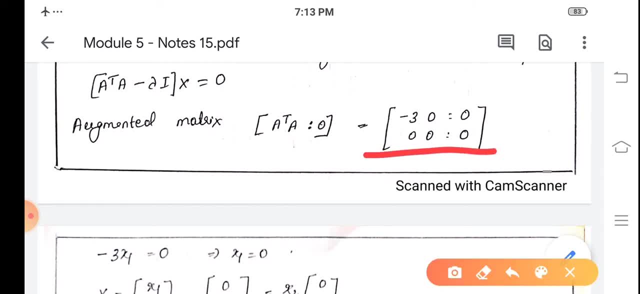 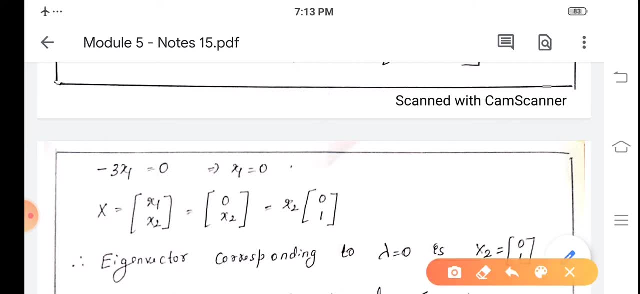 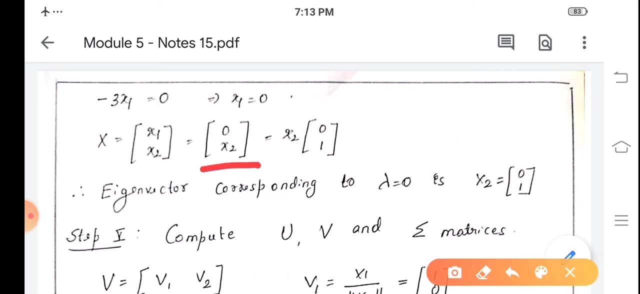 We have the equivalent´s value of aτ x, But since lambda equal to 0, League matrix is A transpose A, 0.. A transpose A is or 0. So we write the equation as: x1 ye A transpose A is 0. 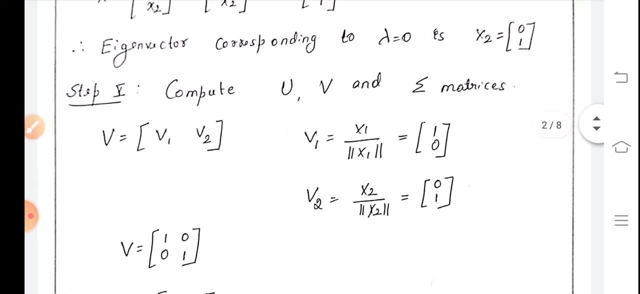 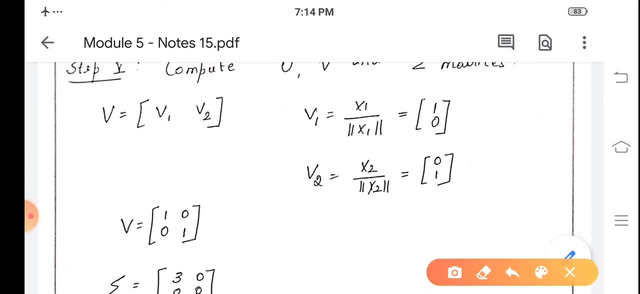 equal to 0, 1. in the next step we find matrices u, v and sigma, where v equal to v 1, v 2 and v 1 is x 1 by norm x 1, v 2 is x 2 by norm x 2. that is v 1 equal to 1, 0, v 2 equal to 0, 1. so matrix v is: 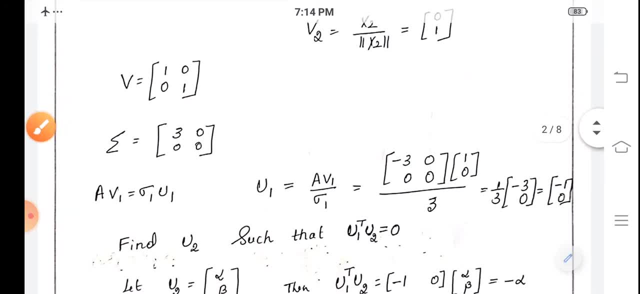 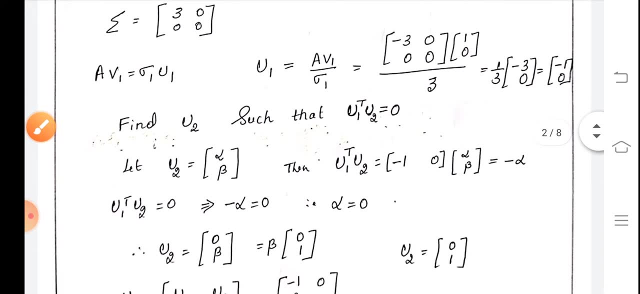 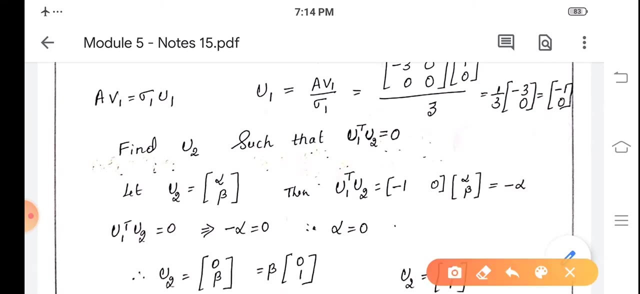 first column: 1, 0. second column: 0, 1. now we write sigma matrix. sigma matrix is 3 0 0, 0 and we need to find matrix u. to find matrix u, here we have a v 1 equal to sigma 1, u- 1. that gives u 1 equal to. 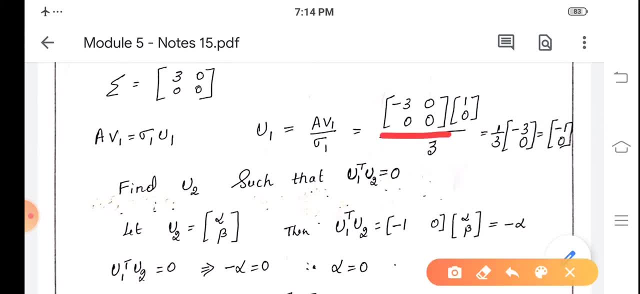 a, v 1 by sigma 1. a is the given matrix minus 3, 0, 0, 0 multiplied by v 1. v 1 is 1, 0 divided by sigma 1. that is the first singular value. 3, that gives 1 by 3 into minus 3, 0 or minus 1, 0. next we need to: 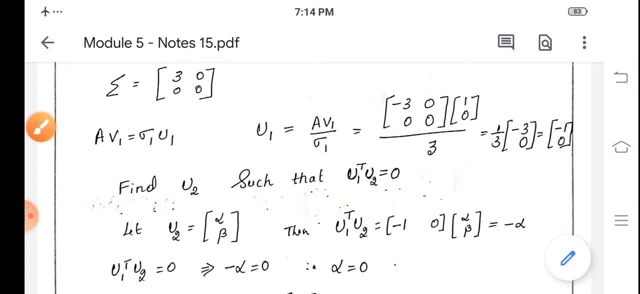 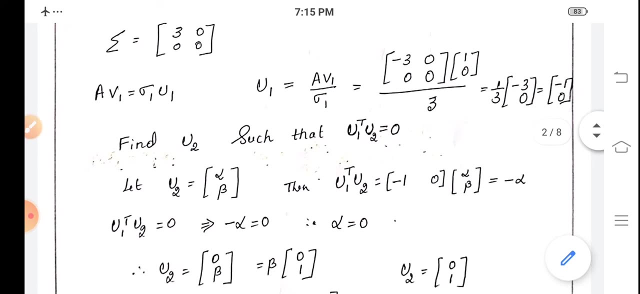 find vector, vector, vector u 2, such that u 1 transpose u 2 equal to 0, because u 1 and u 2 are orthogonal and we take u 2 equal to alpha beta. so since u 1 and u 2 are orthogonal, u 1 transpose u 2 equal to 0. that gives 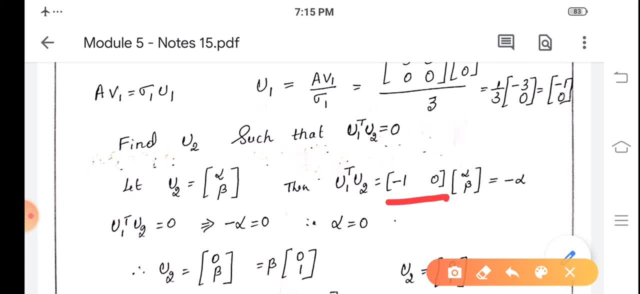 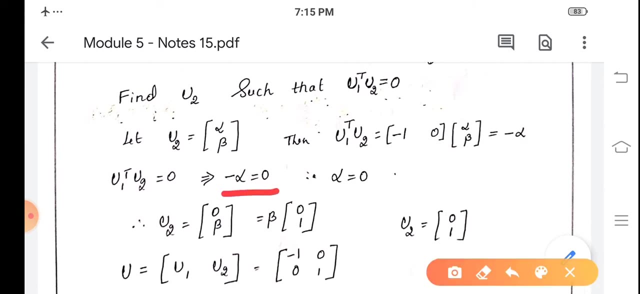 u 1 transpose u 2 is minus 1: 0. row vector minus 1: 0. multiplied by u 2, u 2 is alpha beta, that is minus alpha. so u 1 transpose u 2 is minus alpha. so since u 1 transpose u 2 is 0 minus alpha equal to 0, that gives alpha. 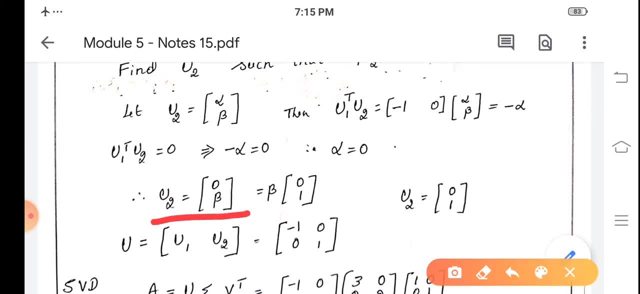 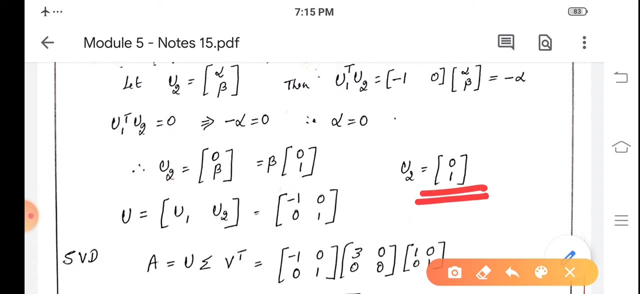 equal to 0. so we write: u 2 is equal to alpha beta, that is 0 beta, so beta into 0, 1. so here we require unit vectors. so u 2 is 0, 1. so this is also unit vector because length of this is. 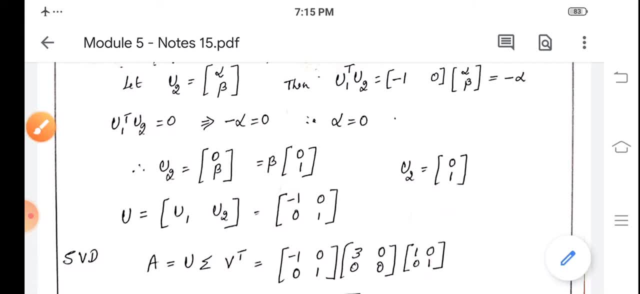 root of 0 plus 1 square, that will be 1. so we need to find vector u. 2 is 0, so this is also unit vector. So we can write vector: u is equal to u1, u2, where u1 is minus 1, 0 and u2 equal to 0, 1.. 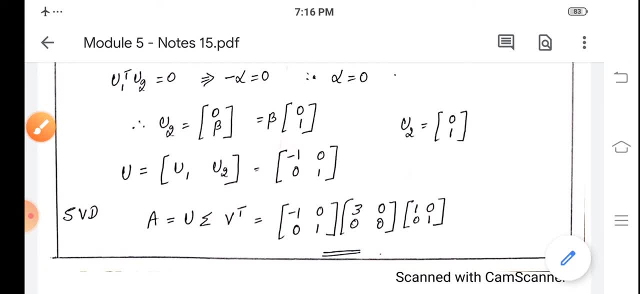 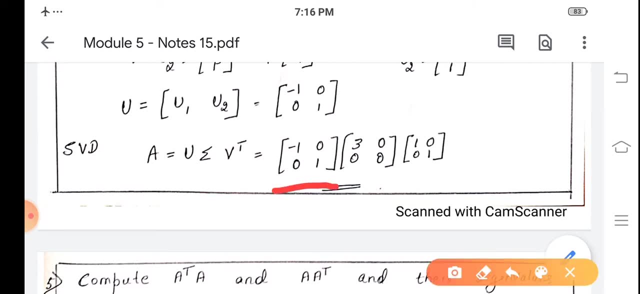 So after getting u, v and sigma matrix, we write the singular value decomposition as a is equal to u sigma v. transpose that is minus 1, 0, 0, 1 into sigma 3, 0, 0, 0 multiplied by v transpose. 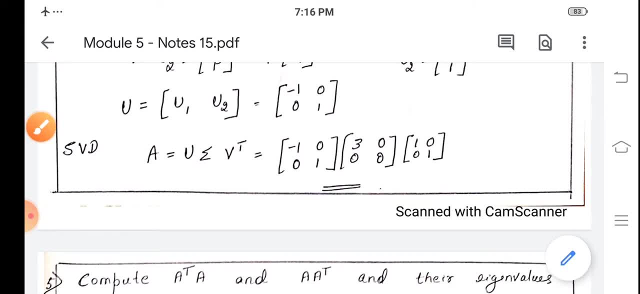 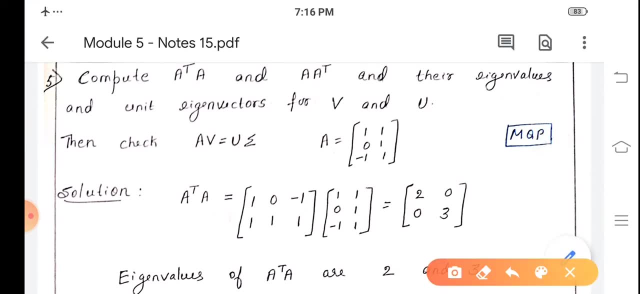 It is transpose of v, that is 1, 0, 0, 1.. Now let us work out the last question. It is question number 5.. Compute a transpose, a and a, a transpose and their eigenvalues and unit eigenvectors for v and u. Check that a into v equal to u into sigma where a is first. 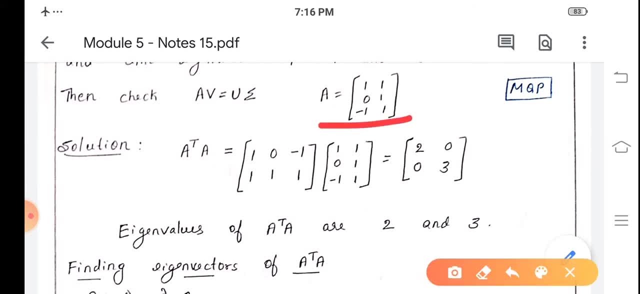 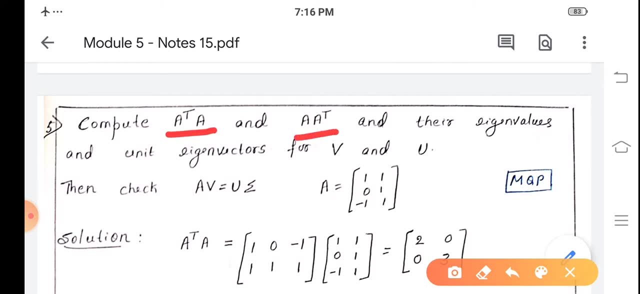 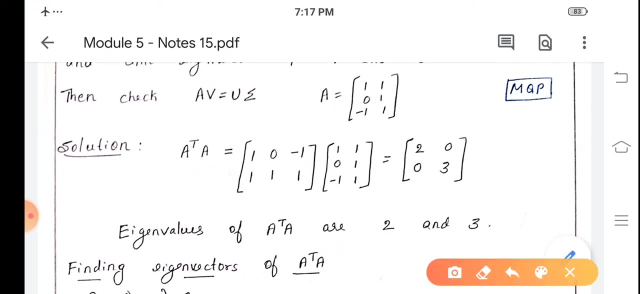 row 1, 1,. second row: 0, 1,. third row: minus 1, 1.. Here we need to find eigenvalues and unit eigenvectors of a transpose a and a a transpose. So first let us find a transpose a. a transpose a equal to a transpose a is 1, 0, minus 1, 1, 1, 1. 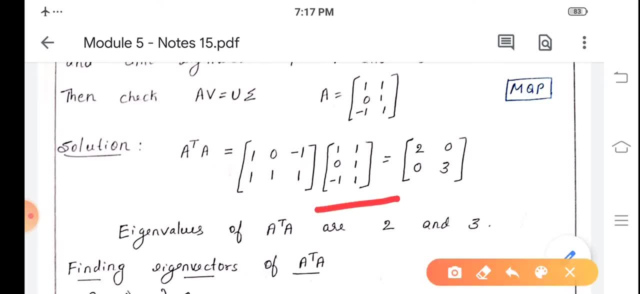 multiplied by given matrix, that is 1, 1,, 0, 1, minus 1, 1, that is 2, 0,, 0, 3.. So a transpose a is triangular matrix. So here the eigenvalues are 2 and 3, because we know that the matrix is triangular. 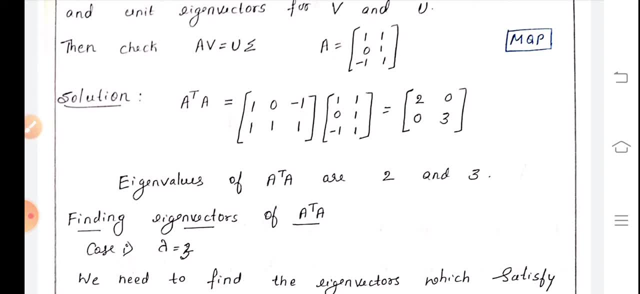 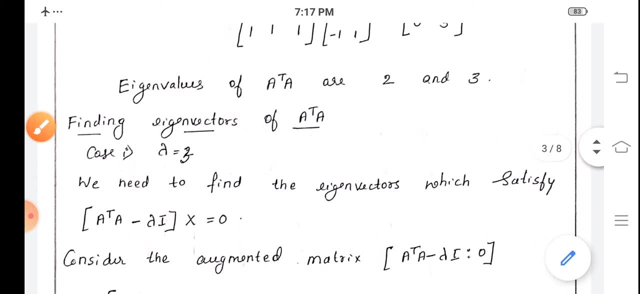 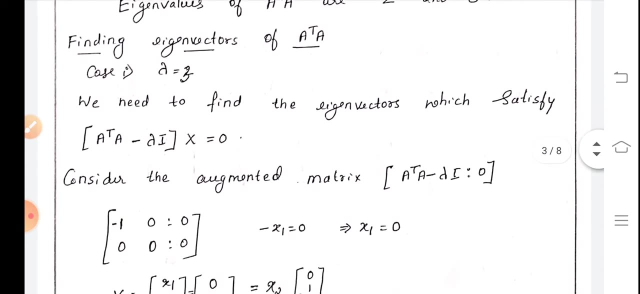 matrix. then the eigenvalues of a triangular matrix are its diagonal entries. So here the diagonal entries are 2 and 3.. So eigenvalues are 2 and 3.. Now we find the eigenvectors of a transpose a. So first case we take lambda equal to 3 and we 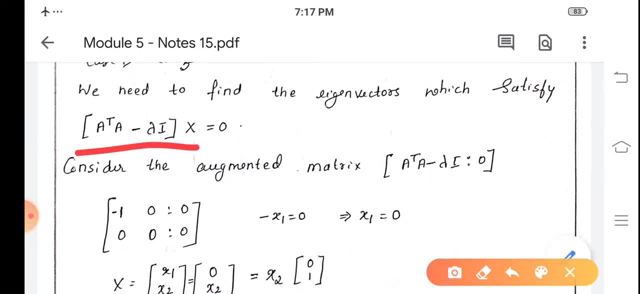 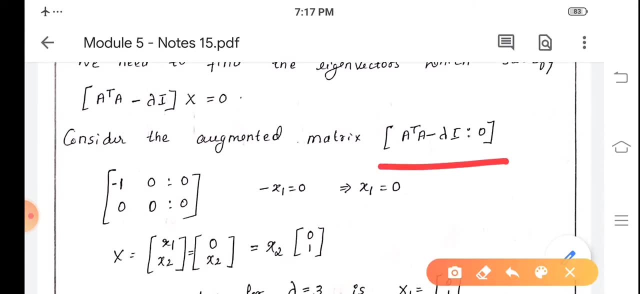 need to find the eigenvectors that satisfy a transpose a minus lambda i into x equal to 0. But since lambda equal to 3, the augmented matrix is a transpose a minus 3 i 0, that will be minus 1, 0, 0, 0, 1.. 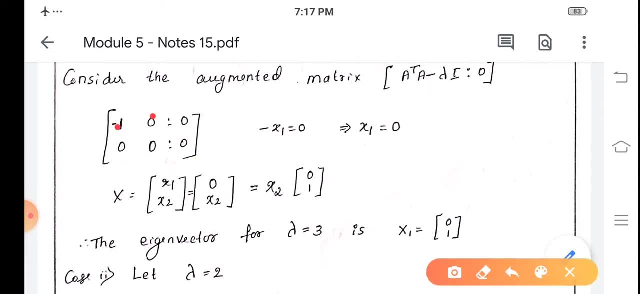 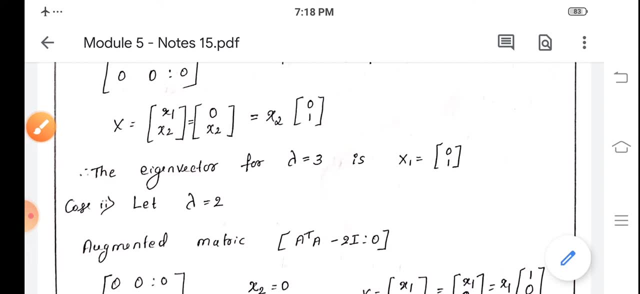 So we can write minus 1 into x1 plus 0, x2 equal to 0. that gives x1 equal to 0.. Now x equal to column vector x1, x2, that is 0, x2. or we write it as x2 into 0, 1. So eigenvector for lambda equal to. 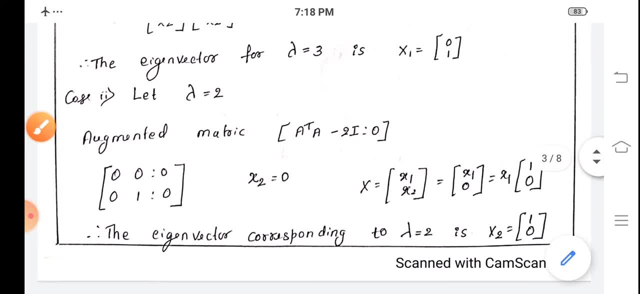 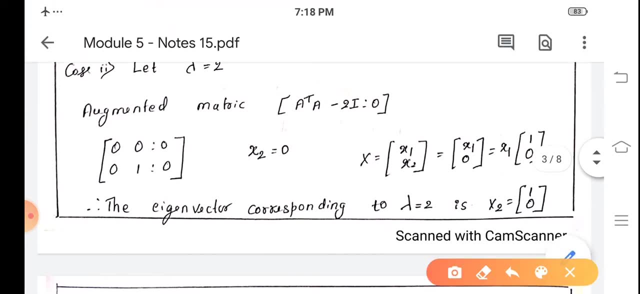 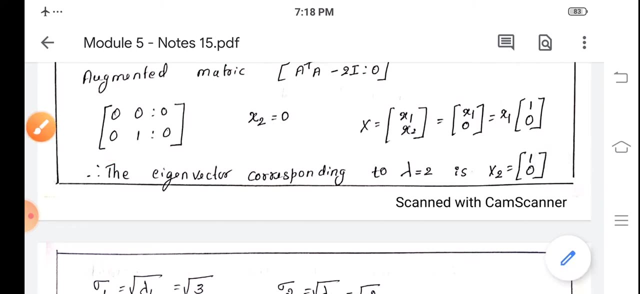 3 is x1 equal to 0, 1.. Next we find the eigenvector for lambda equal to 2.. For lambda equal to 2, we take augmented matrix as a transpose, a minus 2 i 0. That is 0, 0, 0, 0, 1, 0.. So multiplying the second row by column vector x, x1, x2,. 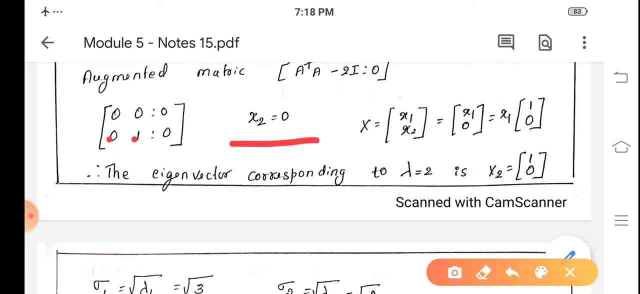 we obtain 0 into x1 plus 1 into x2 equal to 0. that gives x2 equal to 0. So x is x1, x2 and it is x1, 0 that gives x1 into 0, 1.. So eigenvector for lambda equal to 2 is x2 equal to 1, 0.. Now 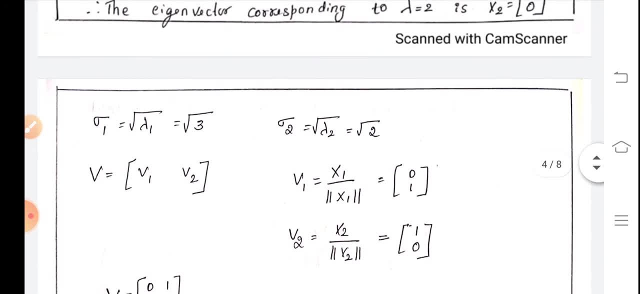 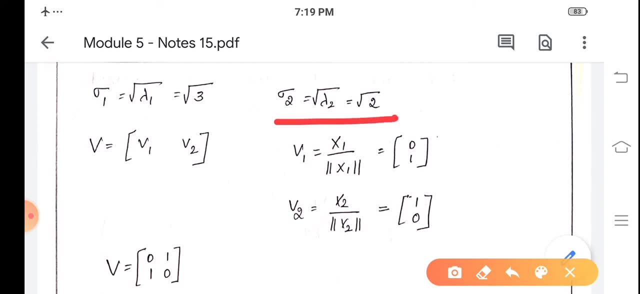 we write the singular values. Singular values are: sigma 1 equal to root lambda 1, root lambda 1 is root 3 and sigma 2 equal to square root of lambda 2, that is root 2.. So we write vector v as v is. 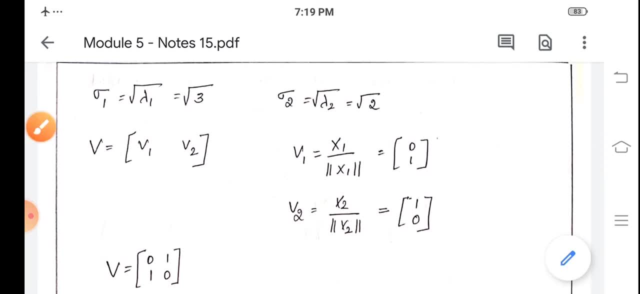 equal to first column v1, second column v2, where v1 is a x1 by norm x1 and v2 is x2 by norm x2.. That will be: v1 is column vector 0, 1 and v2 equal to column vector 1, 0. So we write vector v as v. 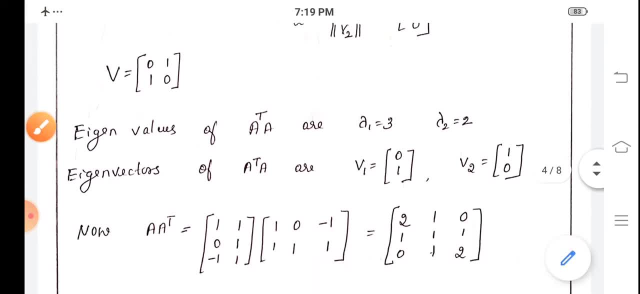 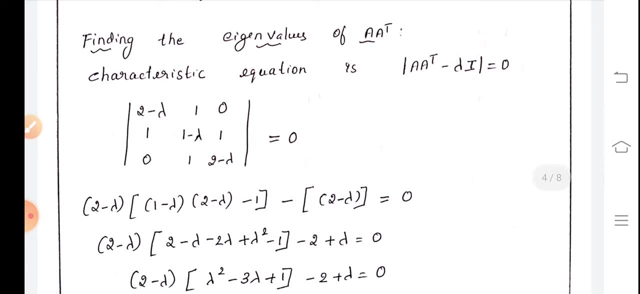 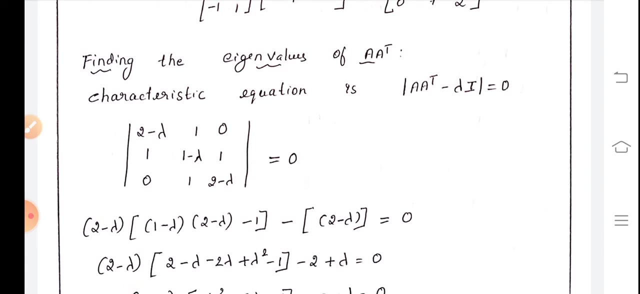 equal to first column 0, 1,. second column 1, 0.. Now, next, we find eigenvalues and eigenvectors of a. a transpose Here to find the eigenvalues and eigenvectors. to find the eigenvalues of a. 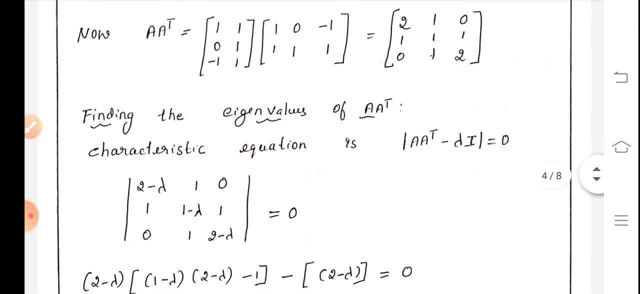 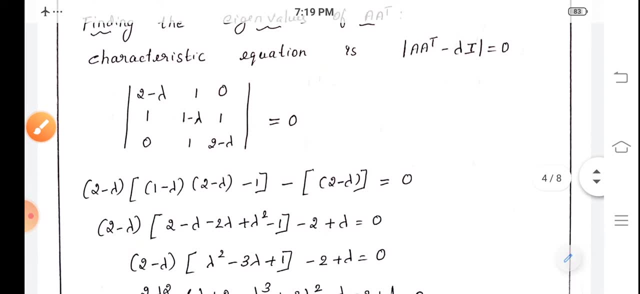 a transpose, we require characteristic equation. The characteristic equation is a a transpose minus lambda determinant 0.. The characteristic equation is determinant of 2 minus lambda 1, 0.. 1, 1 minus lambda 1, 0. 0,. 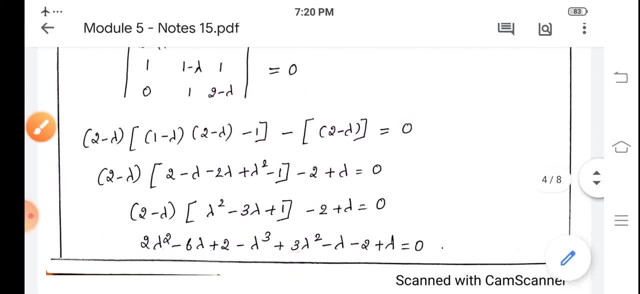 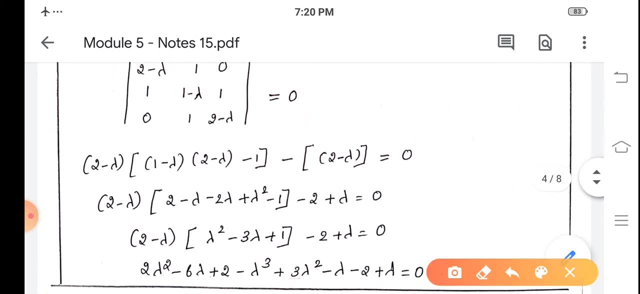 1, 2 minus lambda equal to 0. So, on expanding this, we write 2 minus lambda into 1 minus lambda, into 2 minus lambda minus 1 minus of 2 minus lambda equal to 0. So on simplifying this, 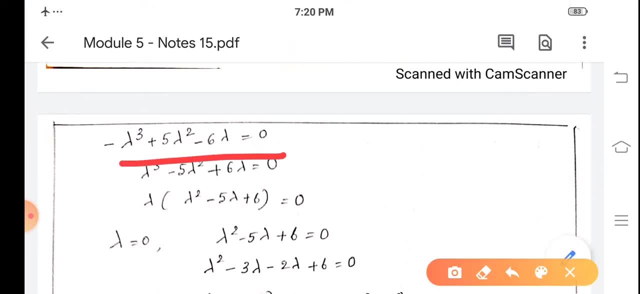 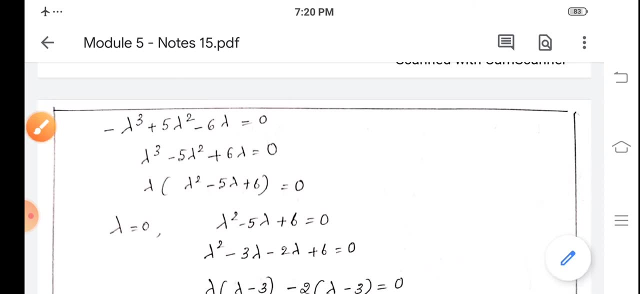 we obtain minus lambda cube plus 5 lambda square minus 6 lambda equal to 0, that is, lambda cube minus 5, lambda Plus 6 lambda equal to 0, or lambda into lambda square minus 5 lambda plus 6 equal to 0.. So on. 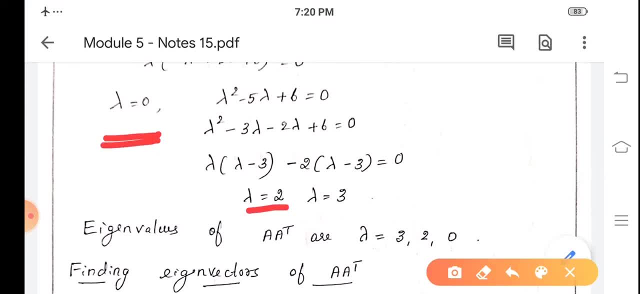 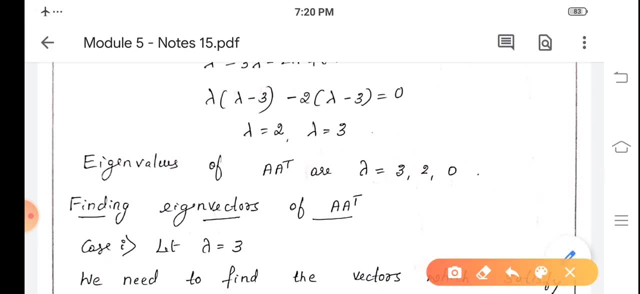 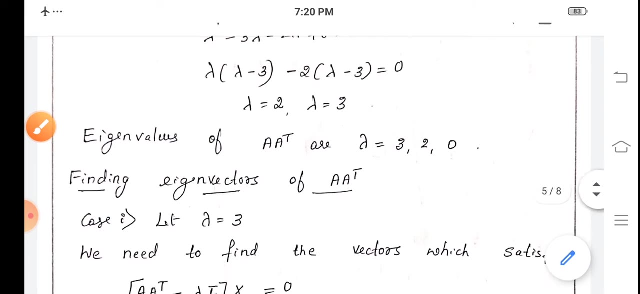 solving this, we obtain 3 values, that is, lambda equal to 0, lambda equal to 2 and lambda equal to 3.. We write these values in decreasing order. So eigenvalues are lambda equal to 3, next lambda equal to 2 and lambda equal to 0.. Next we need to find the eigenvectors of a, a transpose. So. 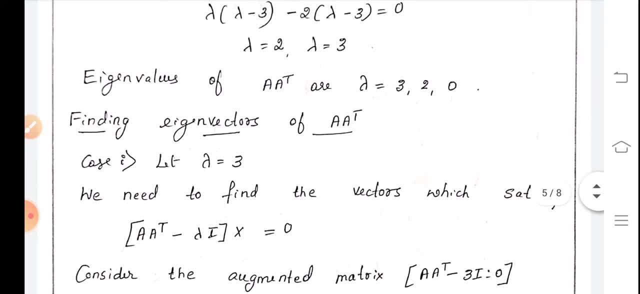 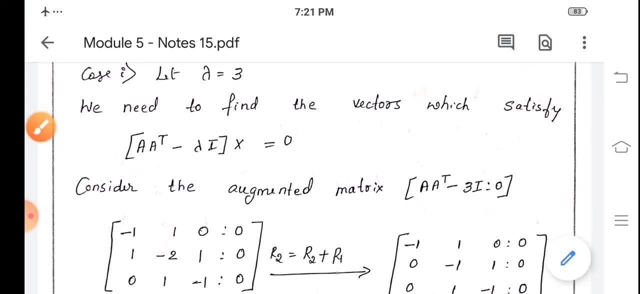 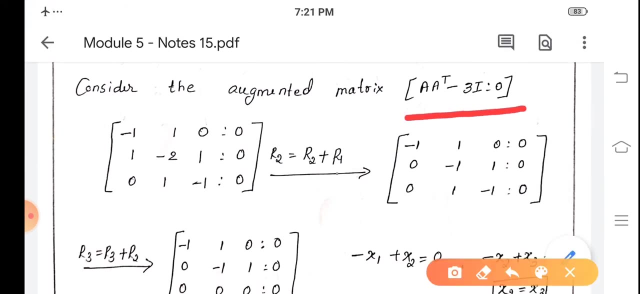 we need to find the unique eigenvectors. First case: we find the eigenvectors of a? a transpose minus lambda i into x equal to 0.. The augmented matrix is a? a transpose minus 3 i 0- that is first row- minus 1, 1, 0, 0, 1 minus 2, 1, 0, 0, 1 minus 1,. 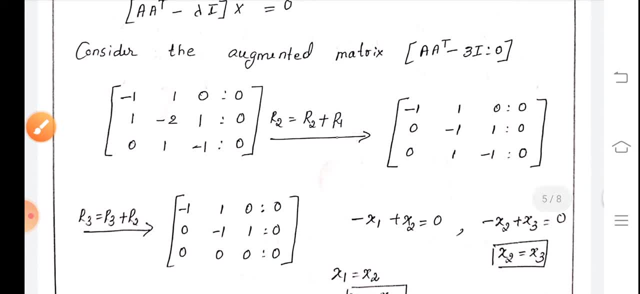 0.. To find the eigenvector, we reduce this augmented matrix to echelon form by writing row operation. Here we write the row operation for the second row operation. So we write the second row as R2 is equal to R2 plus R1.. That will be minus 1, 1, 0, 0, 0,. minus 1, 1, 0, 0, 1,. 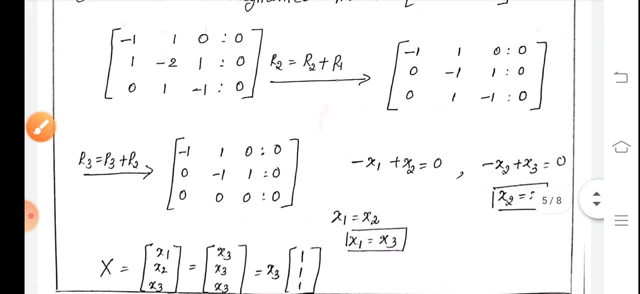 minus 1, 0.. So in order to get echelon form, we require one more row operation. That is for the third row. it is R3 is equal to R3 plus R2.. Now we obtain minus 1, 1, 0, 0, 0,. minus 1, 1, 0, 0, 0,. 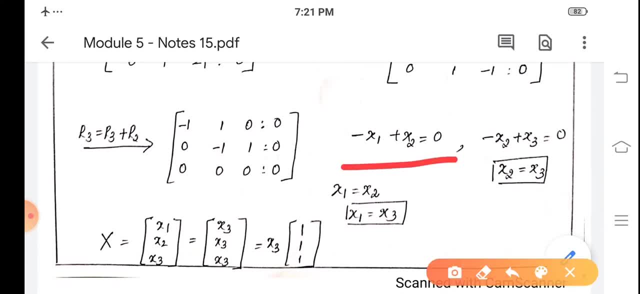 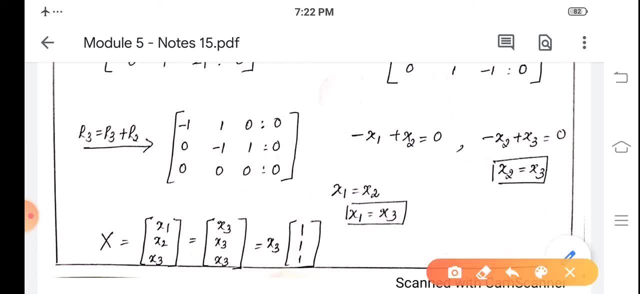 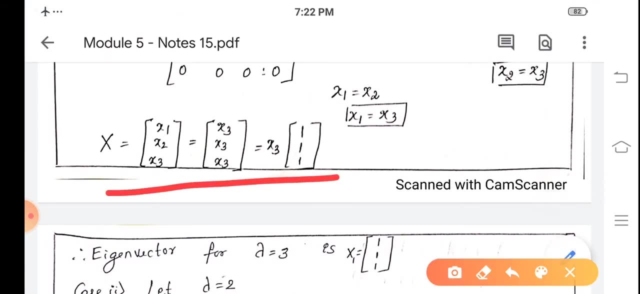 equal to 0. that gives x2 equal to x3. now, using this in the first equation we can write x1 equal to x3. therefore the eigenvector is x1, x2, x3, that is x3, x3, x3 or x3 into 1: 1: 1. so eigenvector for: 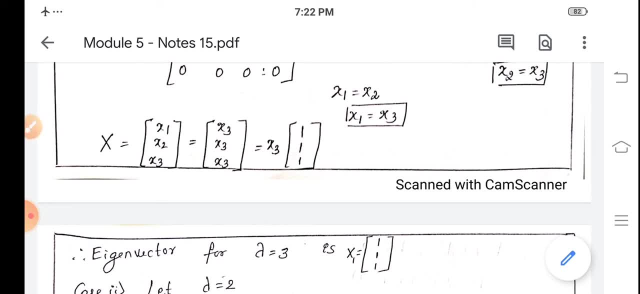 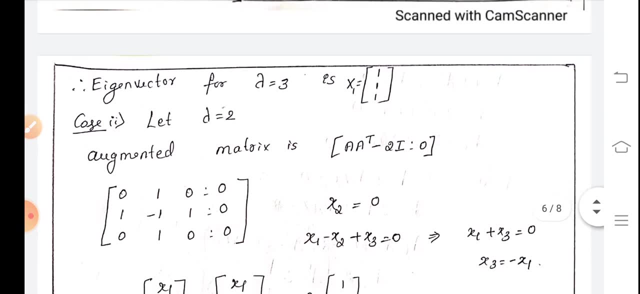 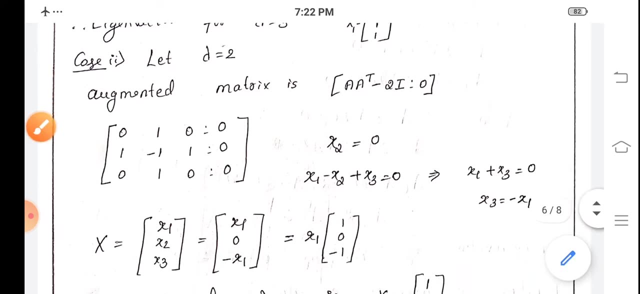 lambda equal to 3 is x1 equal to 1, 1, 1. next, in the second case, we take lambda equal to 2. now we write the augmented matrix as a, a, a transpose minus 2y, 0, that is 0, 1, 0, 0, 1 minus 1, 1, 0, 0, 1 0, 0. 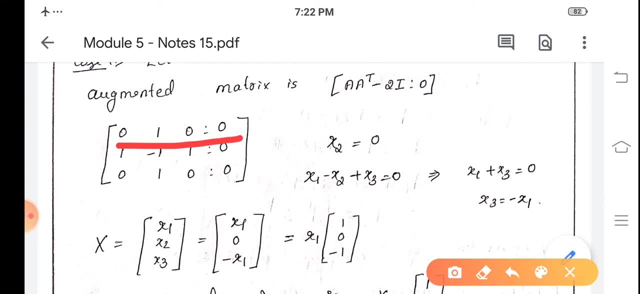 so if we multiply the first row with column vector x, we write 0 into x1 plus 1 into x2 plus 0 into x3 equal to 0. that gives x2 equal to 0.. By multiplying the second row with column vector x, we obtain x1 minus x2 plus x3 equal to 0. that is, x1 plus x3 equal to 0 or x3. 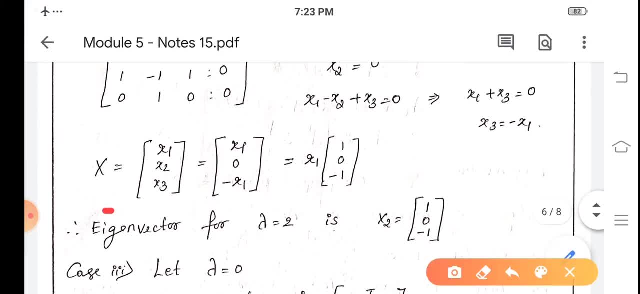 equal to minus x1.. So now we obtain x equal to x1, x2, x3, that is x1, 0 minus x1, or x equal to x1 into 1, 0 minus 1.. So eigenvector for lambda equal to 2 is x2 equal to 1, 0 minus 1.. 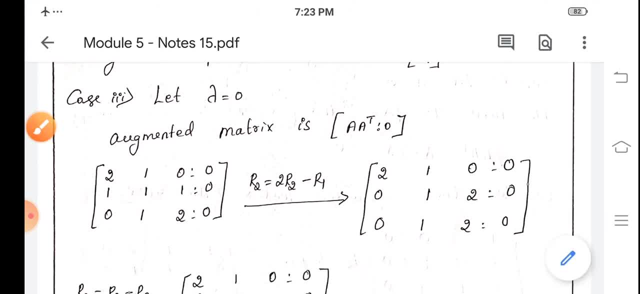 Next we take the last case, that is, lambda equal to 0. and for lambda equal to 0 we write the augmented matrix as a a transpose 0. that will be 2 1 0 0. 1 1 1 0 0, 1 2 0.. Then we write the row. 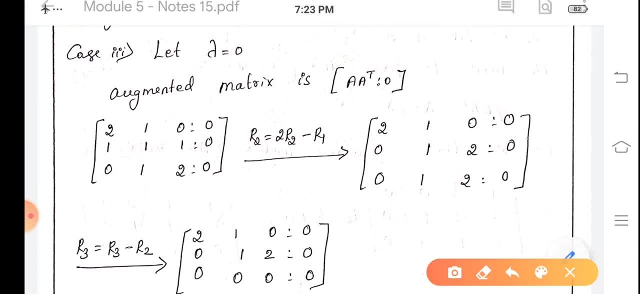 operation for the second row to. in order to get epsilon form, that is r2 equal to 2 times r2 minus r1, that is 2 1 0 0 0. 1 2 0 0, 1 2 0.. So again, we write the row. operation for the last row. 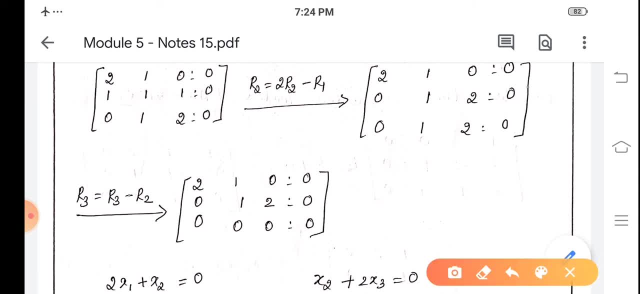 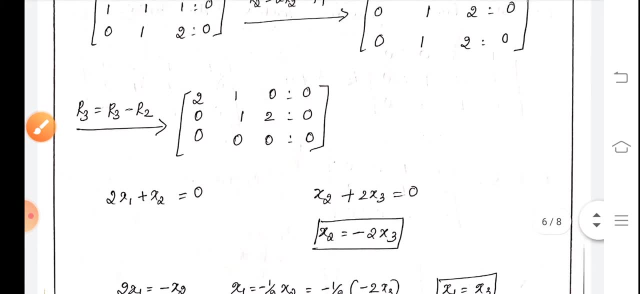 that is r3 equal to r3 minus r2.. So augmented matrix is 2: 1 0 0 0. 1 2 0 0 0, 0.. Here we can write the equation as: 2 x1 plus x2 equal to 0, and by multiplying the second row with column vector. 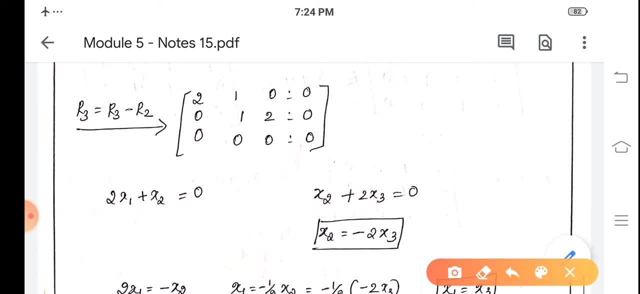 x, we obtain x2 plus x3 equal to x3. equal to x3 minus r2.. So again we write the row operation for lambda: equal to 2 x1 plus 2 x3 equal to 0, that is x2 equal to minus 2 x3.. So using this in the 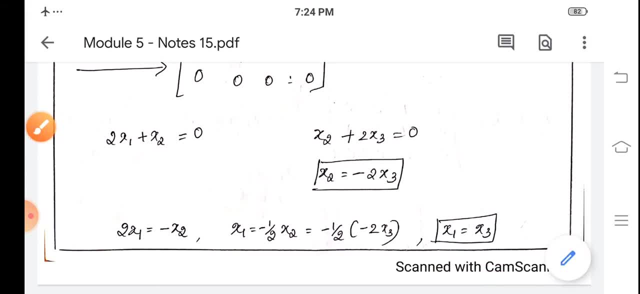 first equation: 2 x1 equal to minus x2, that is x1 equal to minus half x2 minus half into x2 is minus 2 x3. that gives x1 equal to x3.. So eigenvector is x equal to x1, x2, x3, that is x3 minus 2, x3, x3. 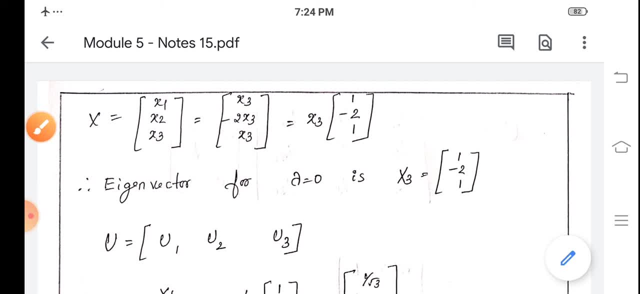 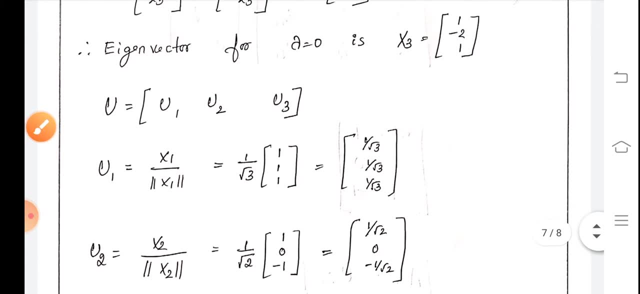 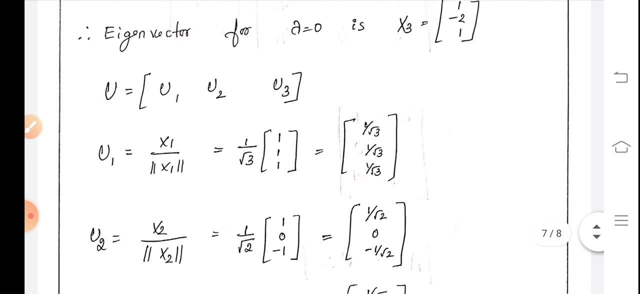 or x3 into 1 minus 2, 1.. So eigenvector for lambda equal to 0 is x3, equal to 1 minus 2, 1. and here we need to find u, where u is equal to u1, u2, u3, that is, u1 is a x1 by norm x1. 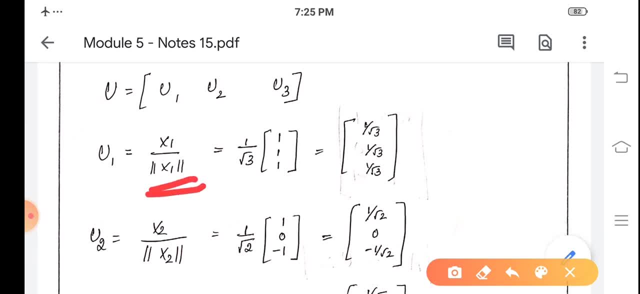 because we require unit vectors. So x1 by norm x1 gives unit vector that is 1 by root 3 into 1, 1, 1, 1 by root 3, 1 by root 3, 1 by root 3. and next u2 is x2 by norm x2, that will be 1 by root 2. 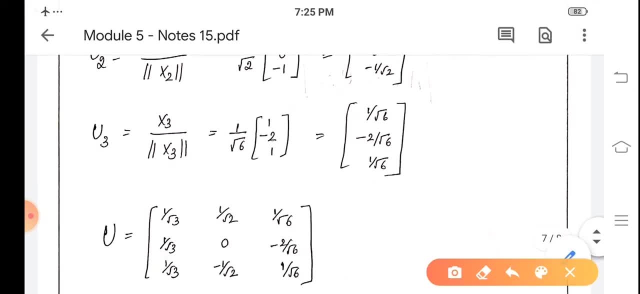 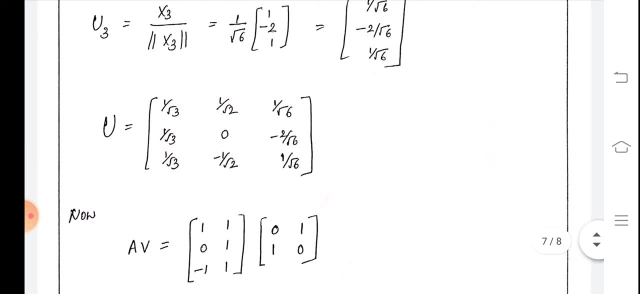 0 minus 1 by root 2. And u3 is x3 by norm. x3, that is 1 by root 6 minus 2 by root 6, 1 by root 6.. So we are getting matrix u as first column: 1 by root 3, 1 by root 3, 1 by root 3, second column. 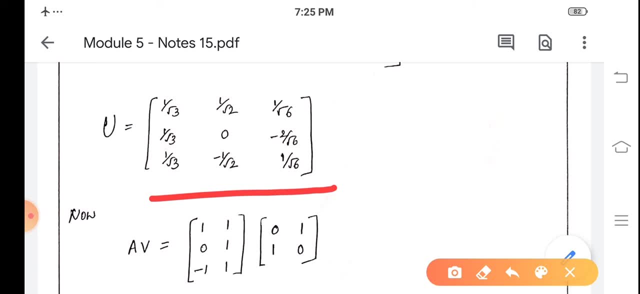 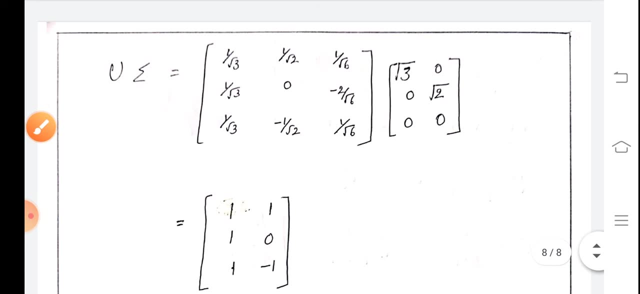 1 by root 2, 0 minus 1 by root 2. and third column is 1 by root 6 minus 2 by root 6, 1 by root 6.. So here we have obtained matrix u, matrix v and also sigma. 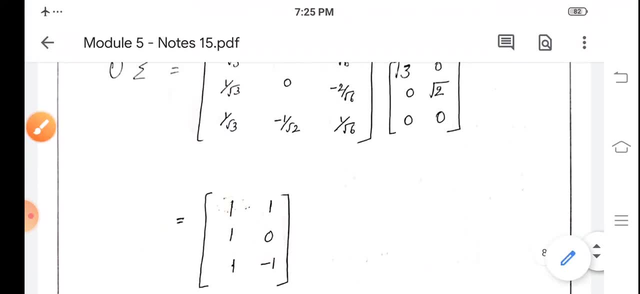 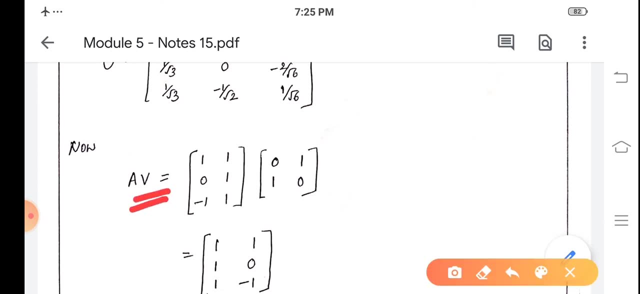 So we have to check av equal To u sigma. now let us find matrix a multiplied by v. a is a given matrix and v is a. a is a given matrix. that is a equal to first row 1, 1, second row 0, 1 and third row minus 1. 1 and v. 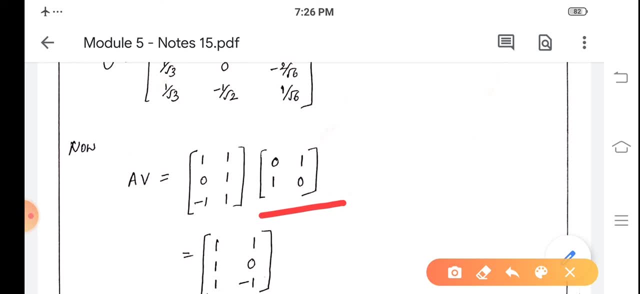 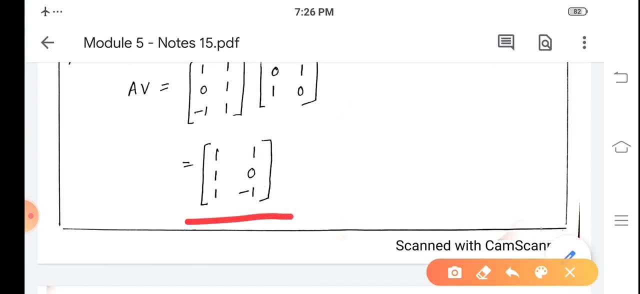 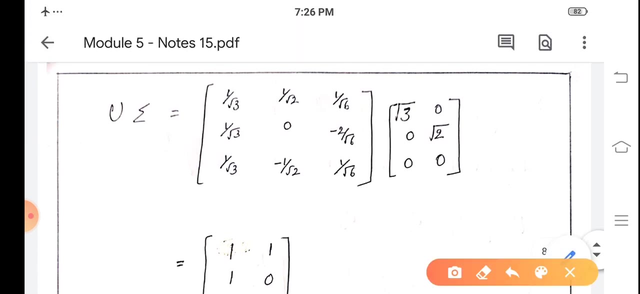 a is a first column 0, 1. already we have calculated v value, that is 0, 1, 1, 0. on multiplying this, we a into v equal to first row 1, 1.. Next we find u into sigma, where u is: first column 1 by root 3. second column 1 by root 3. third: first column 1 by root 3, 1 by root 3, 1 by root 3. second column 1 by root 2, 0 minus 1 by root 2. and third column 1 by root 6 minus 2 by root 6, 1 by root 6 multiplied by sigma. sigma, singular values. 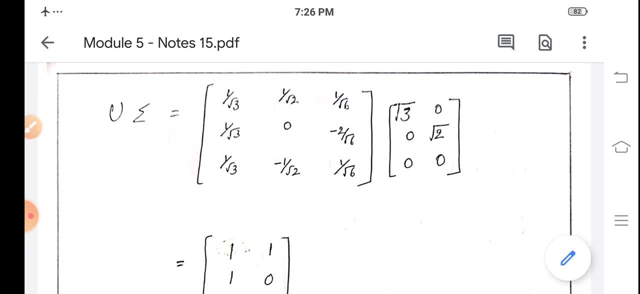 Since the given matrix is of order 3 cross 2, sigma is of order 3 cross 2.. So here Diagonal entries are non-zero singular values, that is root 3 and root 2, and the rest of the entries are zeros. here we can add a column of row of zeros. 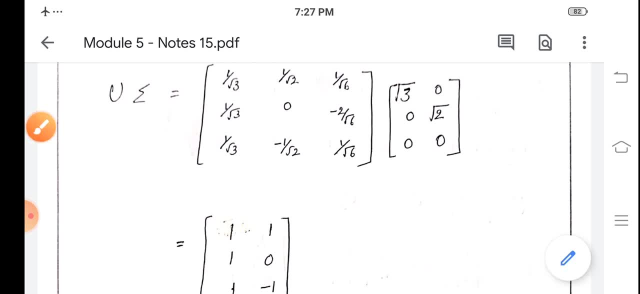 So sigma is root 3 0 0, root 2 0 0. multiplying this we obtain u sigma equal to first row 1, 1, second row 1: 0 and third row 1 minus 1. on comparing av and u sigma: av and u sigma. 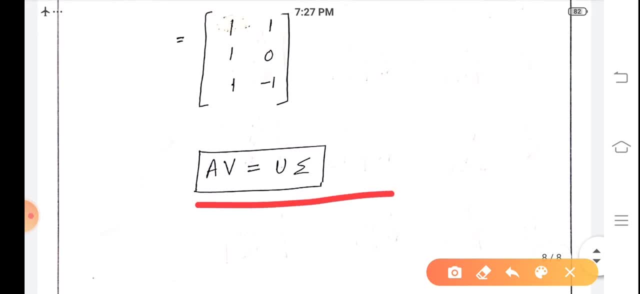 So we can observe that av is equal to u sigma, av is equal to u sigma.